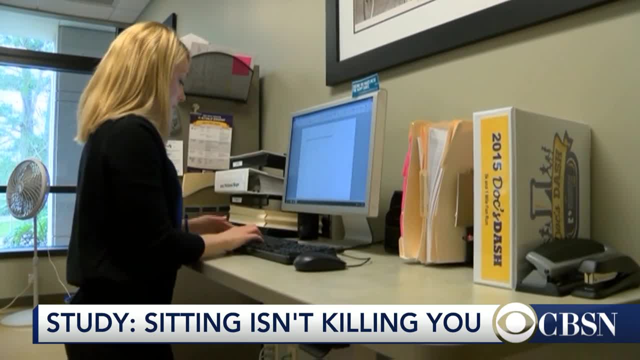 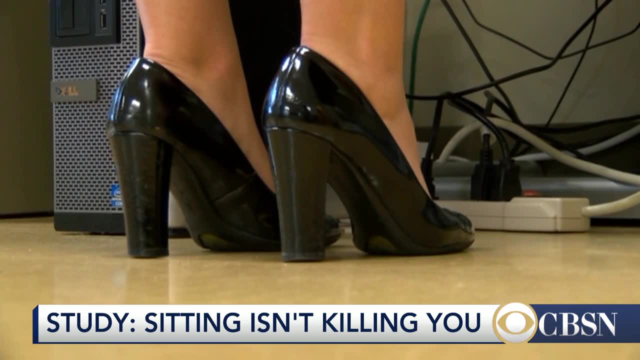 death over those 16 years. Now that goes against some of the studies that we've seen, which show that people who sat more or people who sat less had the same overall risk of death over those 16 years. So we can say that the more you sit, the greater your risk of all causes of death. But we can't.